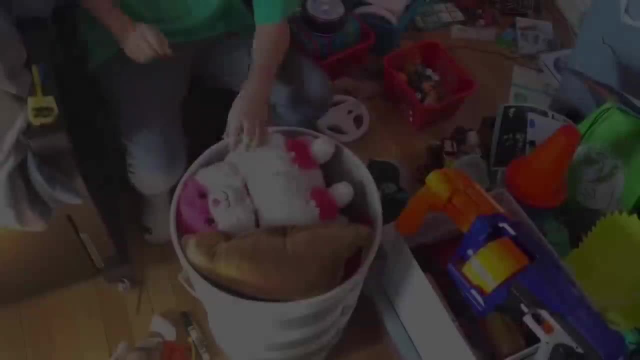 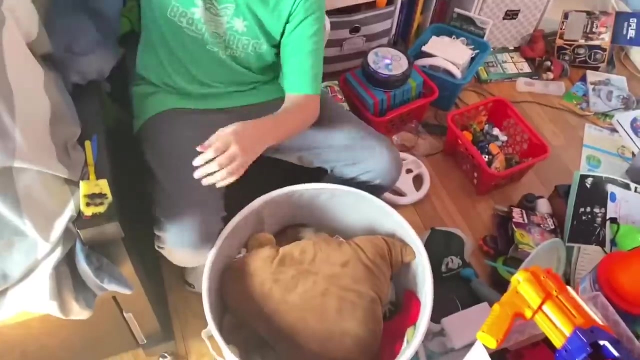 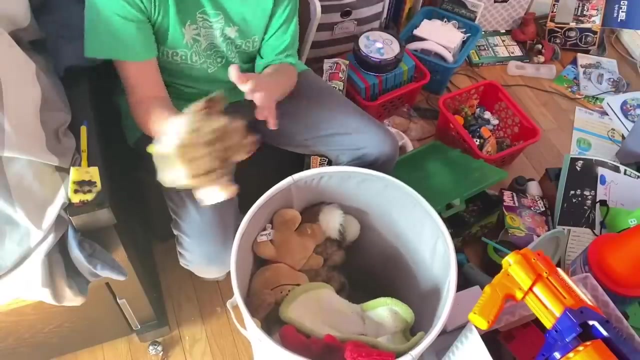 So the reason why I asked Tyler where he wanted to start cleaning up his room is because I wanted him to develop the decision making skills on where to start cleaning up. For my entire life I never knew where to start, so I just avoided it altogether. So if I can empower him by letting 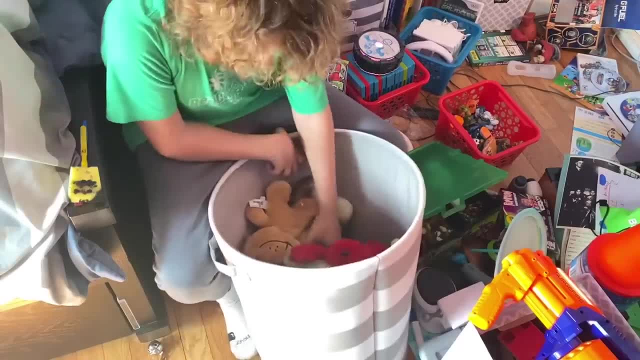 him make the decisions on what he wants to do. that will give him confidence to move forward and find it easy to declutter and give up easily. So now we're talking about cleaning your room. So my answer to that question is this: please start cleaning your room early every time you meet your son and 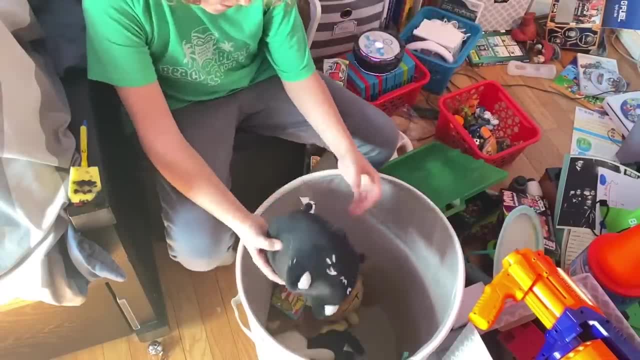 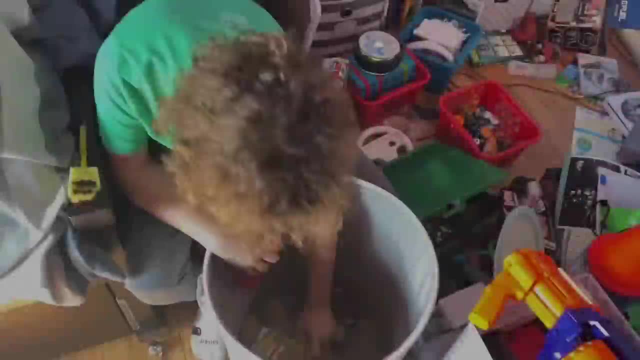 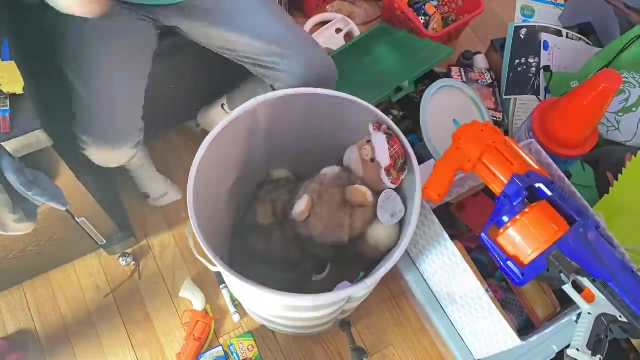 clutter and clean. I was also watching his behavior so that I can also help him be successful, because I noticed with his plushies he didn't want to let anything go. So his plushies were a very sentimental item to him, which means I'm not going to force him to let any of it go. 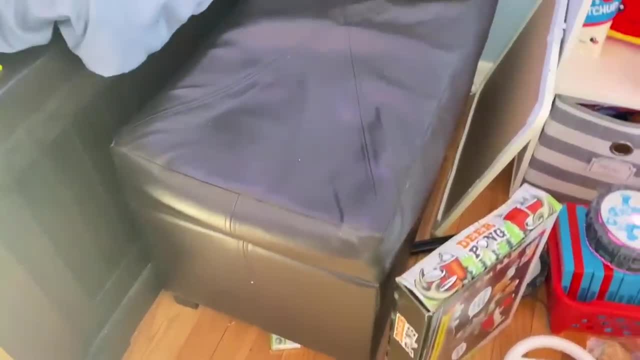 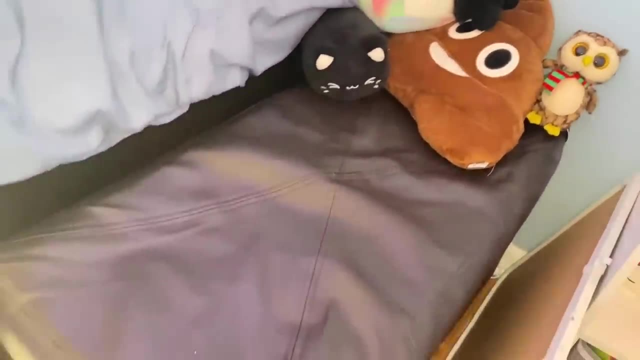 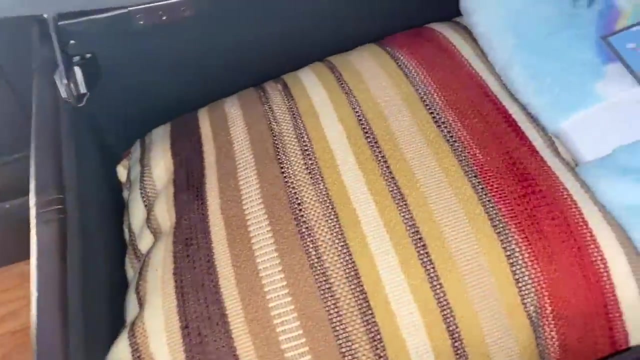 because that would attach a negative stigma if I had forced him to let go of his plushies. Now, this bench right here used to be in our bedroom. When Christmas came, we moved this into his room temporarily, but he actually really liked it and wanted to keep it, So we will have. 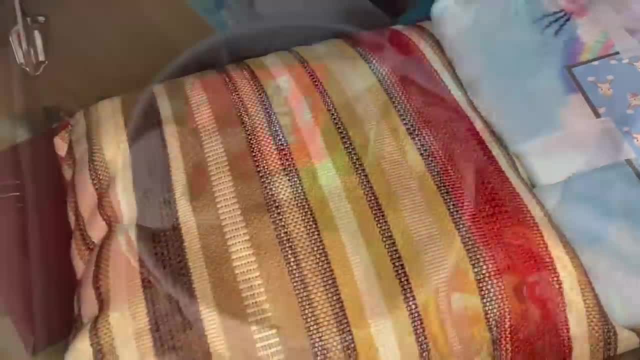 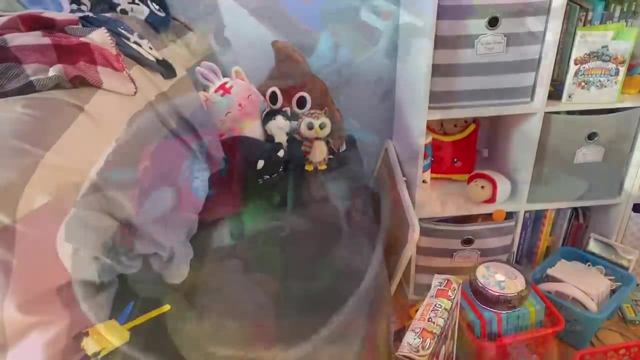 to clean that out, because that's our stuff in there. But the plushie bin used to be in that corner where the bench is, So I think we're going to move the plushie bin to over on this side. So in a little bit we'll declutter some stuff. 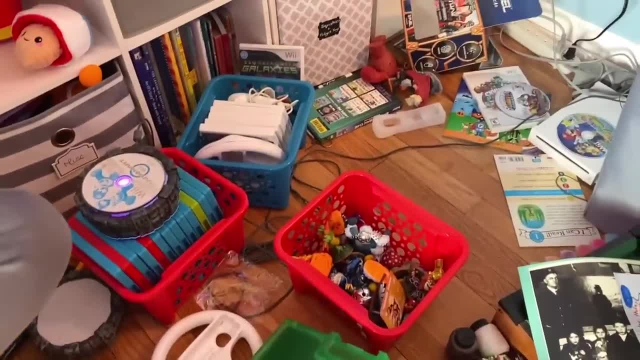 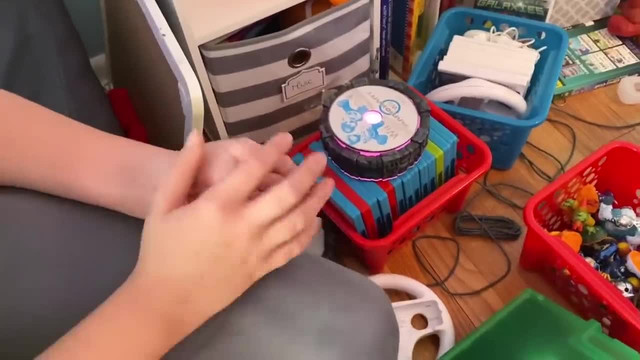 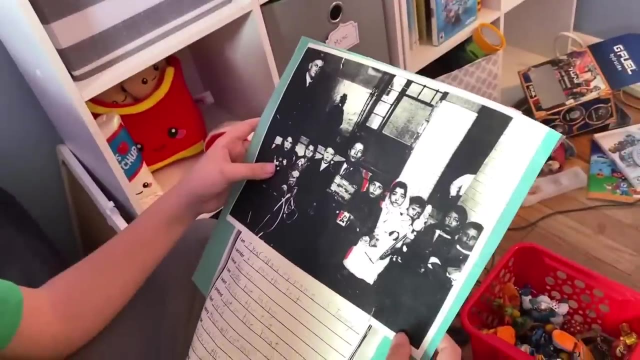 Over there too, because we're going to reorganize all the games. Do you see anything that's trash? Yeah, that's trash, huh, So we can get rid of that. We can find something else. You made that in school. I don't know what this is. I don't know either. You did make it, But what do you? 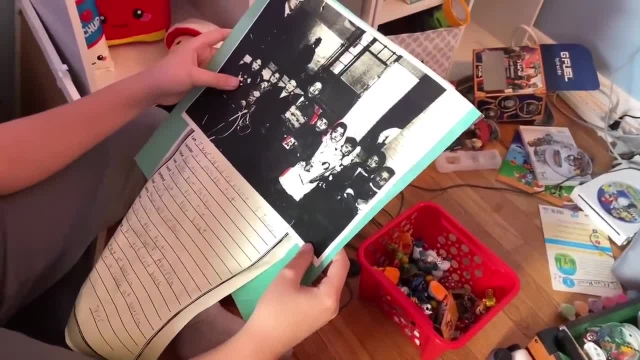 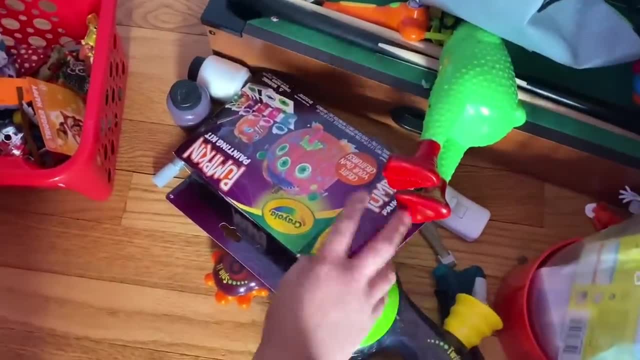 want to do with that. Do you want to keep it or let it go? Let it go. Okay, we can do that. And as we were going through stuff, I just realized that it was just a mixture of stuff that he did want to keep. But 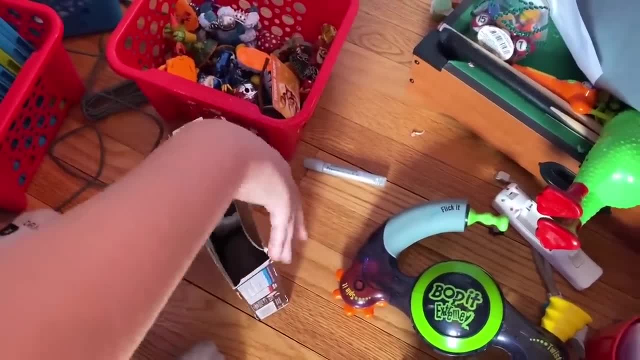 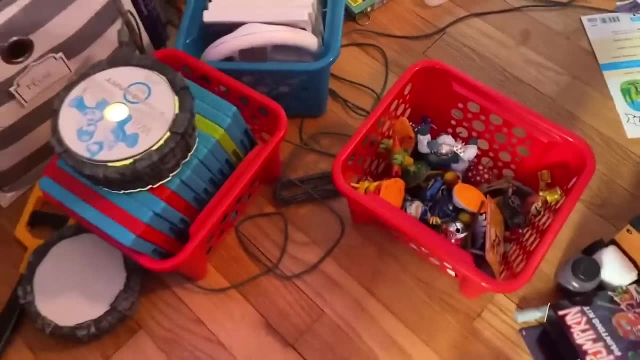 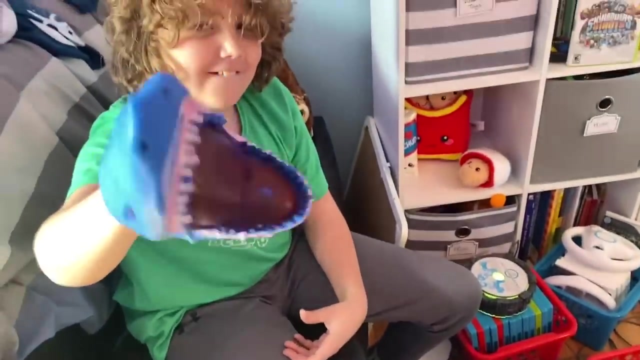 they just weren't categorized. There was art supplies and games and random pieces that just weren't put back. So right now we're just doing some rough categorizing so that he can identify where to put the things back to. My Sharky is going crazy, Sharky, going crazy, Oh, Sharks. 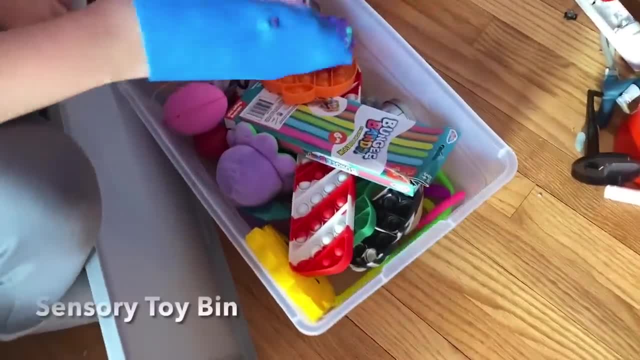 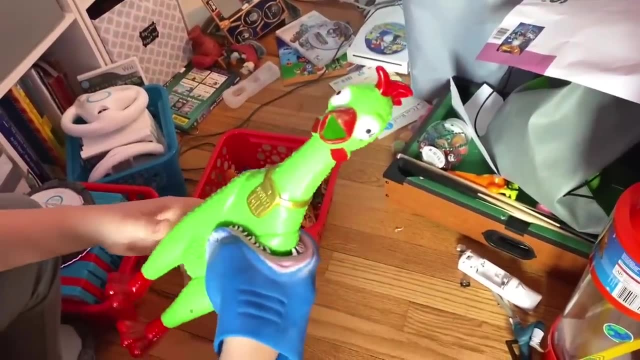 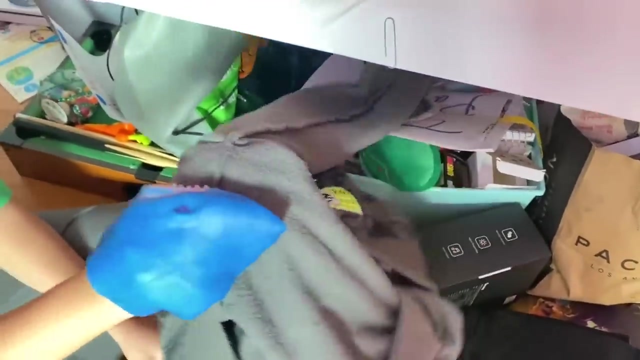 So now Sharky is going to join us on this video in the decluttering and categorizing, because, look, if you can make it more fun for a kid, they will be more eager to finish this up. Because sharky, the decluttering shark, were ready to start putting things where 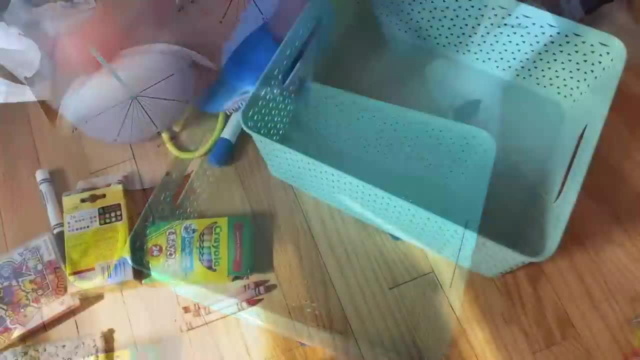 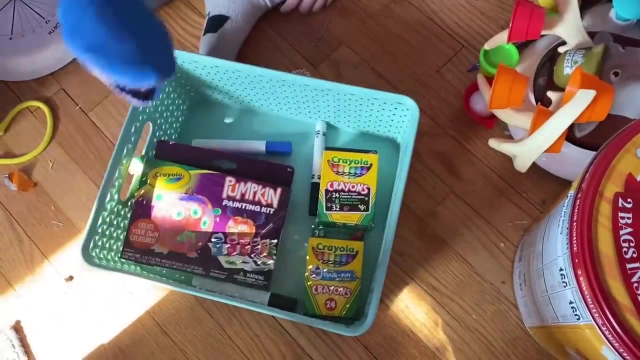 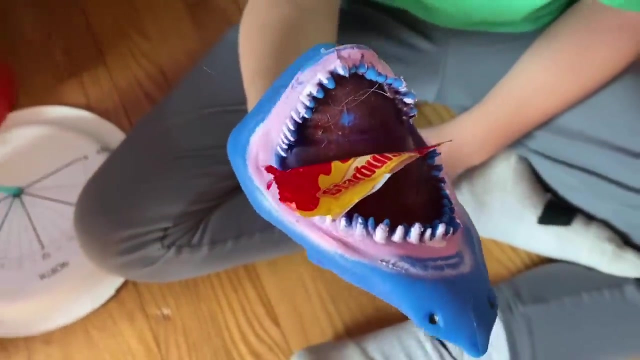 they belong, Start categorizing things like this art bin. Right now, we're just gathering all of the art supplies that we find and just putting them into this bin. Now, Believe it or not, I never did this as a child myself. My parents never forced me to clean up. 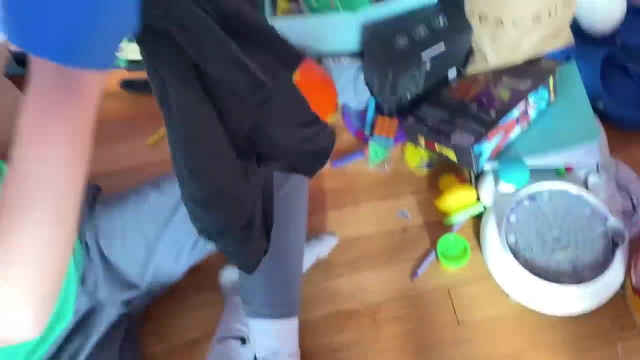 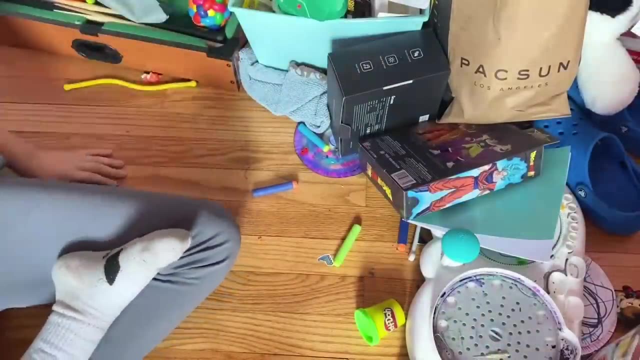 My mother actually felt bad for me because when she was a little girl she didn't clean up, But when she got older she didn't have hoarding disorder. She knew exactly what to do and cleaning and organizing was very natural to her. 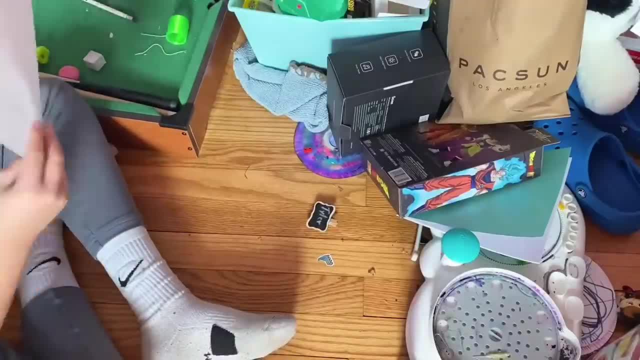 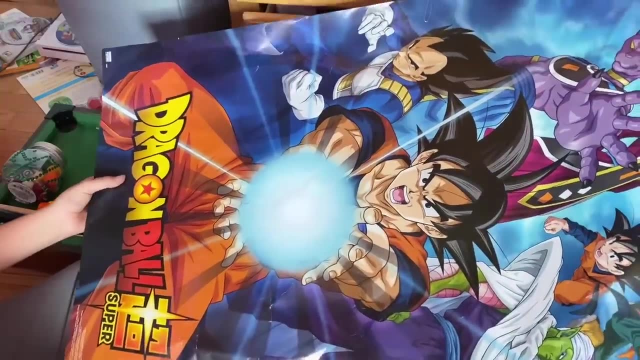 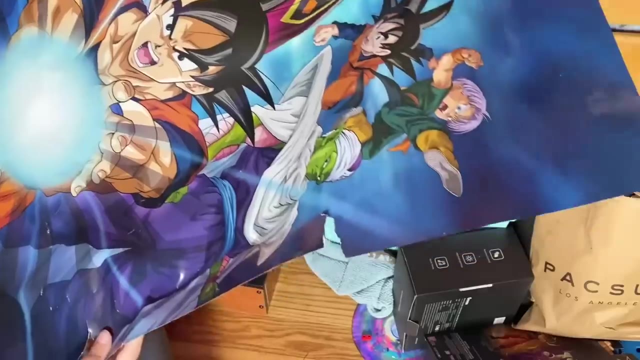 She had no idea that her daughter had the hoarding disorder gene This poster. she got a little ruined, But the good news is that you have the same exact poster, brand new, that we can hang on your wall. So you want to let go of this poster then? 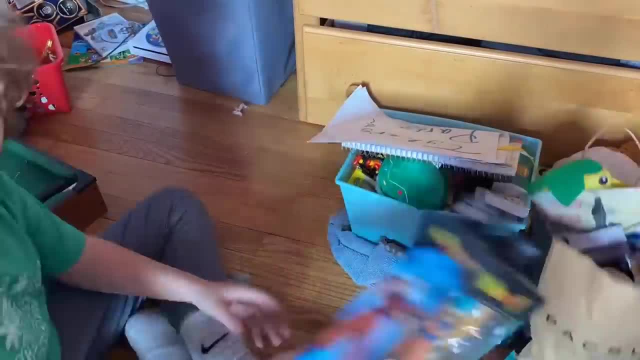 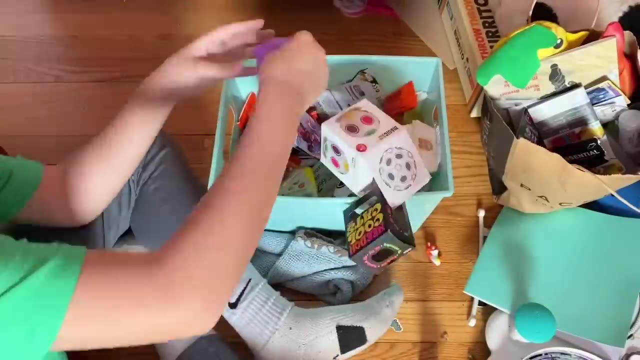 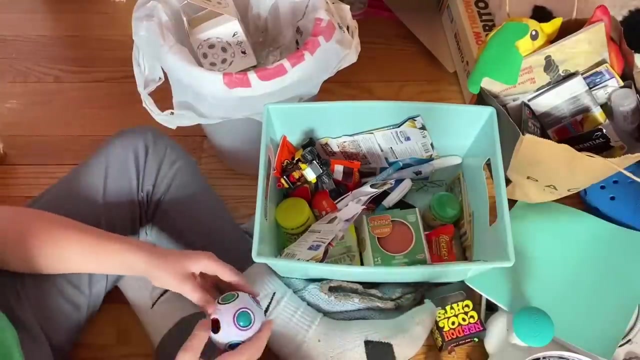 Yeah, This is also the reason why we do the New Spend Challenge each and every month, And we've been very mindful of what we're buying for Tyler. He's only really gotten gifts for his birthday and Christmas, But yet things still come through that door without us buying it. 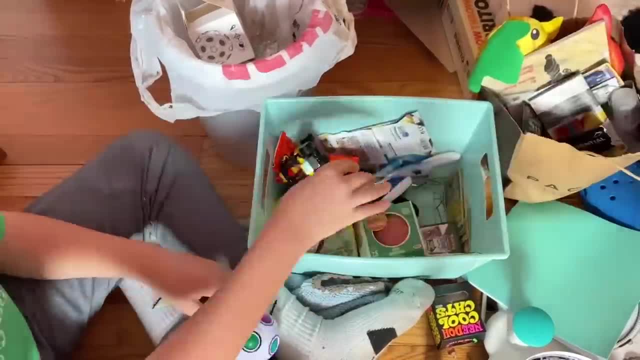 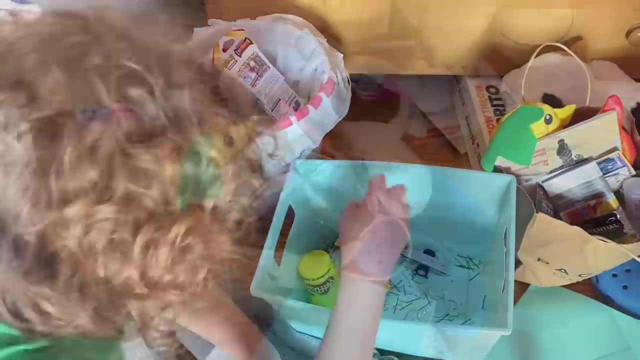 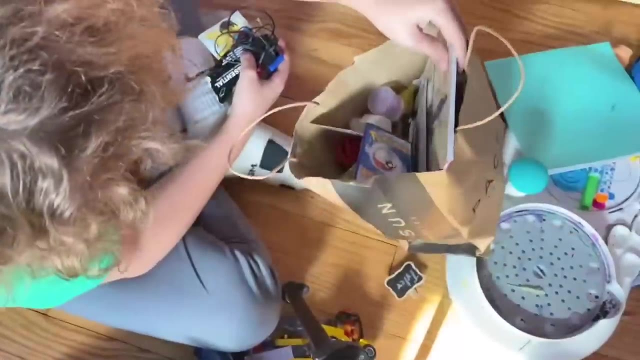 Like gift bags from other children's birthday parties, The prize box from when he does really good in school. Things are always trickling in. I think this bag is a trash bag that we Do. you want to let that go? Are these things in here that we can let go of? 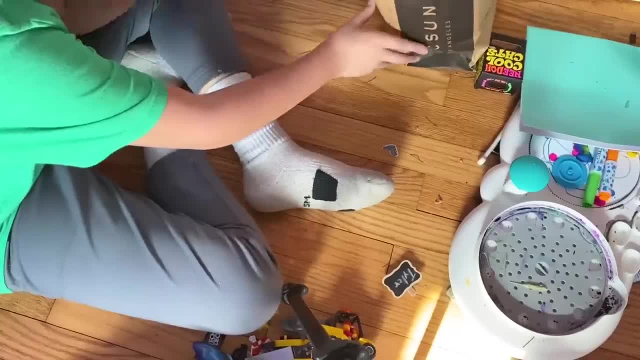 Yeah, that whole bag can go. that's in there Looks like a bunch of random stuff. huh, We're going to let all of that go. Yeah, That whole bag can go. that's in there Looks like a bunch of random stuff. huh, We're going to let all of that go. 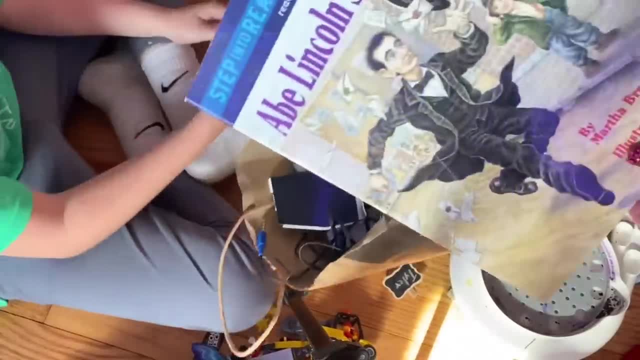 Looks like a bunch of random stuff. huh, We're going to let all of that go. Looks like that's a book, so we'll have to give away that book then. Looks like that's a book, so we'll have to give away that book then. 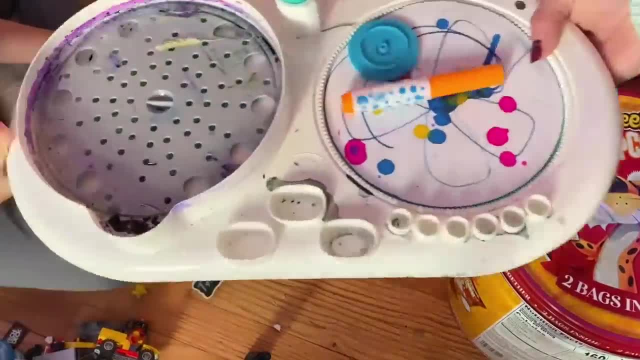 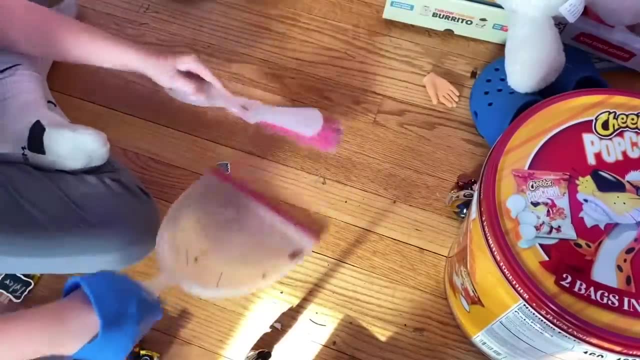 Another thing that we kind of have to bring back is kind of like Fly Lady, but for the kids We were doing good for a real long time And then again, sometime around November, it kind of fell to the wayside. Oh, but what about this? 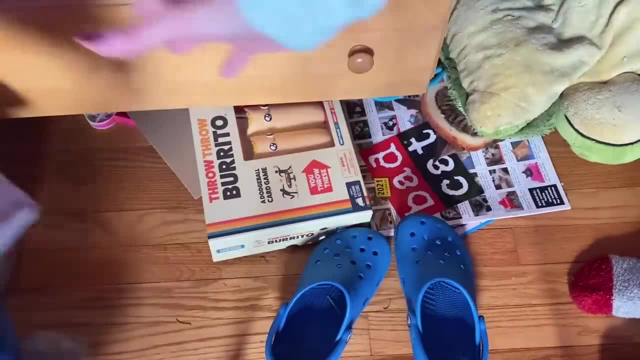 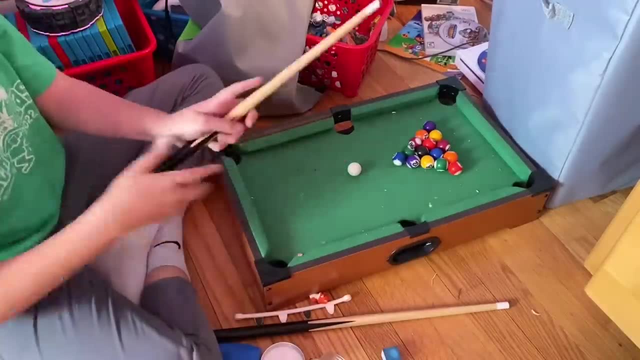 Can we let that go? Yes, we're going to let that go. Uh-oh, Oh, there's more trash in the bag. And since we're identifying where we need to improve, Oh, there's more trash in the bag. 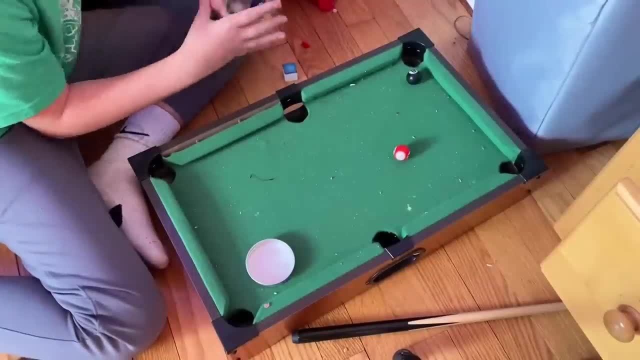 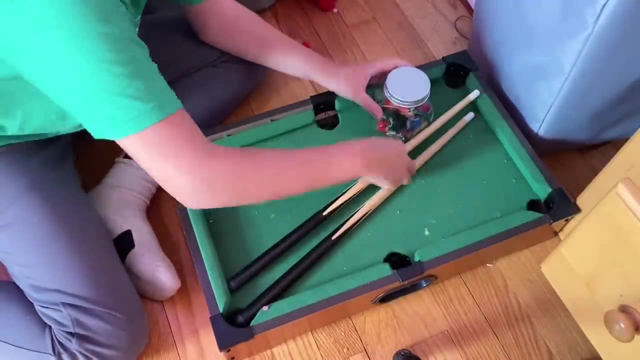 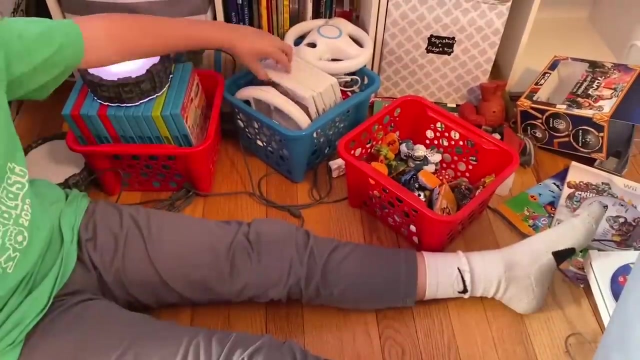 And since we're identifying where we need to improve what works better for us and our behaviors and habits, it's very important to give myself and my children the grace as we learn to declutter better and clean better, Because shaming somebody else that their kids have a messy room or just putting ourselves down that we can't do it. 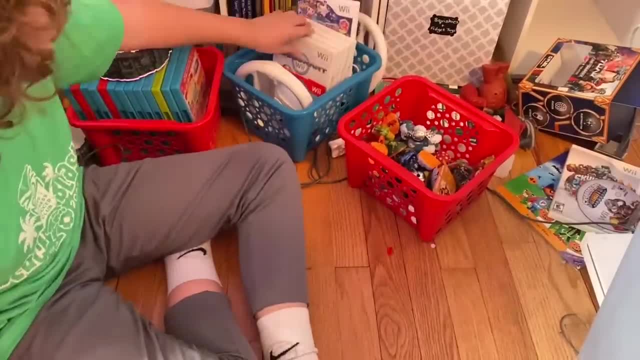 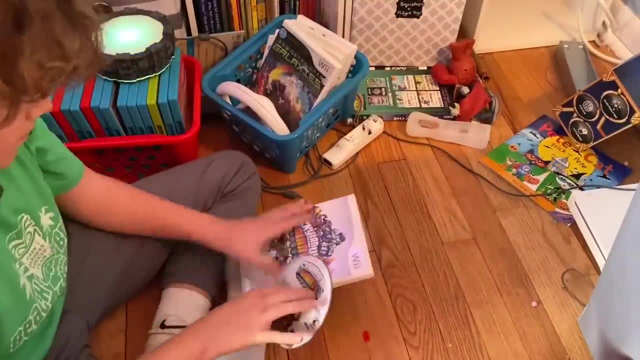 it's not going to be beneficial to anyone. It's okay if the messes came back because- let's be realistic- It's not as bad. It's not as bad as it used to be. The children's room declutter used to be something like over 10 episodes just to declutter it. 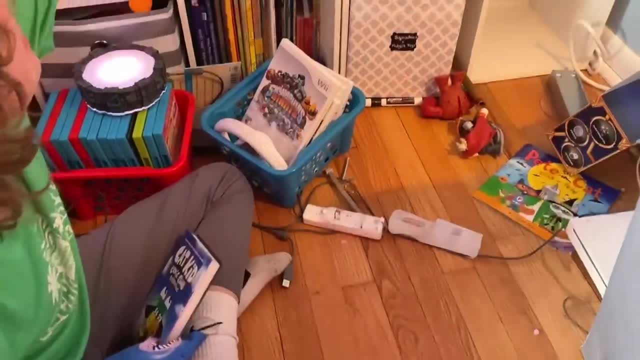 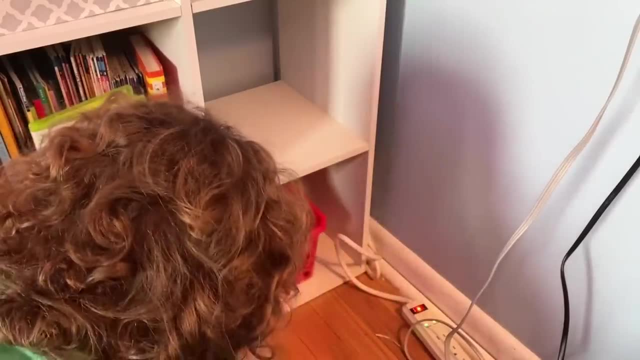 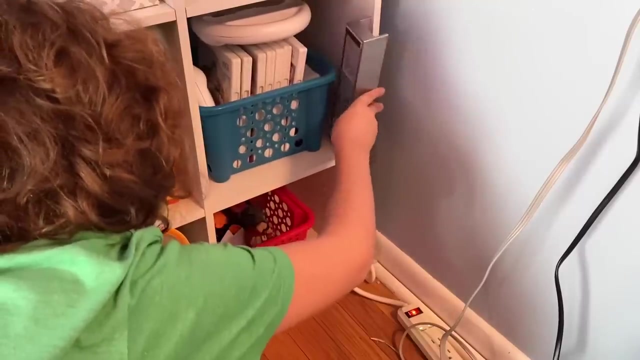 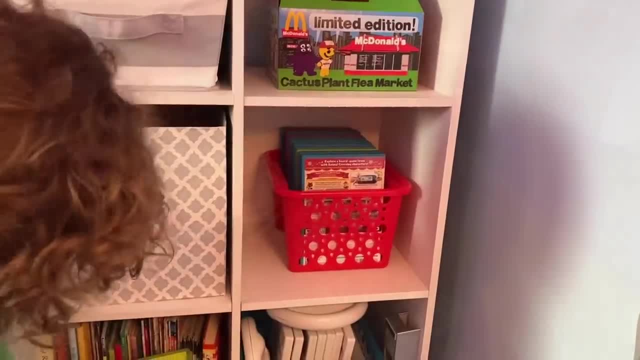 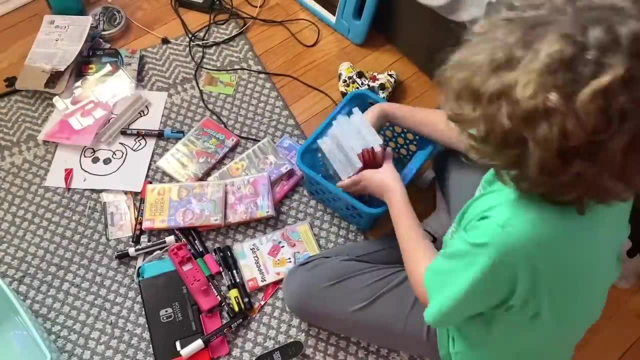 It takes a lot of time. It takes time especially processing emotions so that you can be successful in it, And my hope is that when you demonstrate this to your children and they're watching you reach your goals, it'll motivate and encourage them too, knowing that they don't have to. 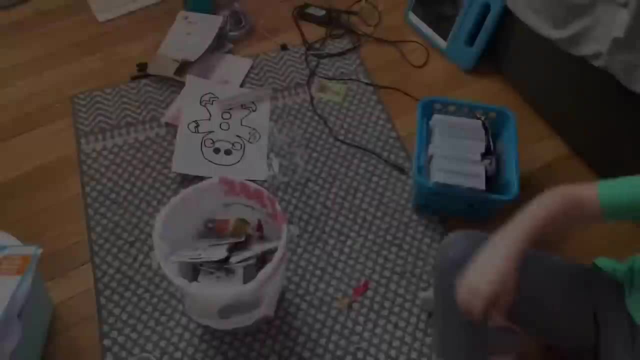 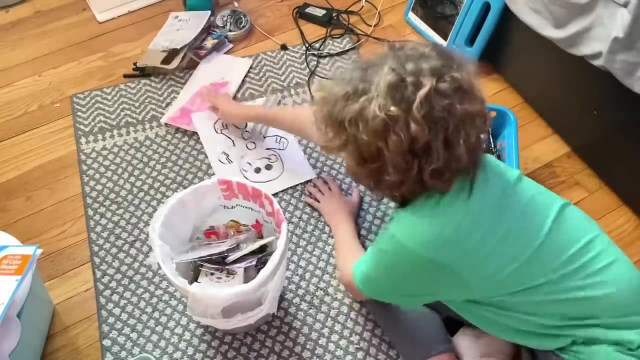 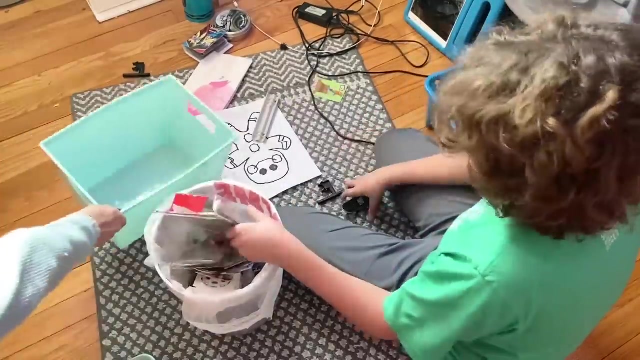 put pressure on themselves and that they can do it too, Because right now, I'm very, very proud of Tyler. He has been putting like with like, identifying what is trash, throwing things And the basic fact that he wants to do it, which means it's a positive experience for. 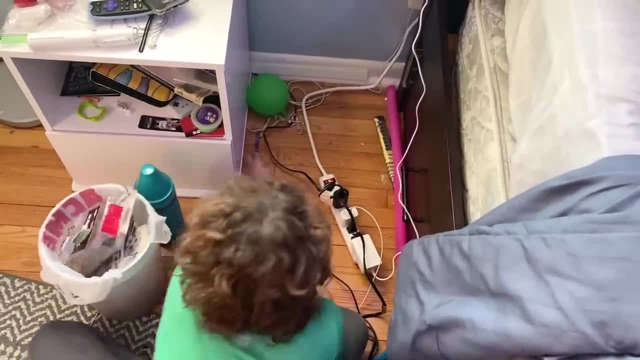 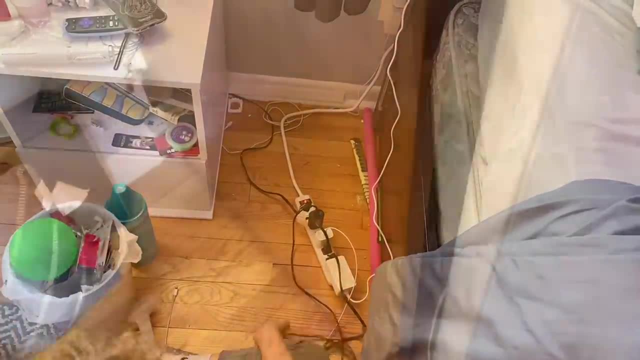 him to do, Because in the end, I don't want either of my boys to end up like a level four hoarder, like their mommy did. I want them to be able to clean with ease. Now Miss Pepper wants to know what on earth is going on in this room. 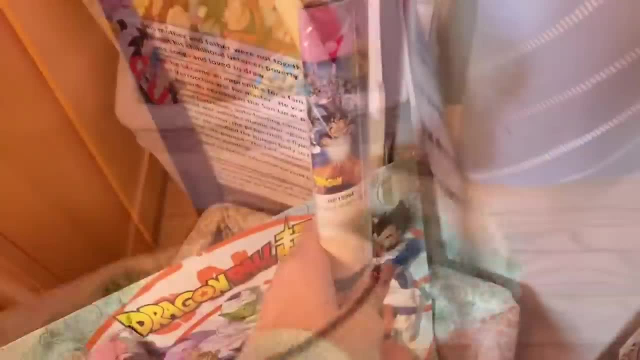 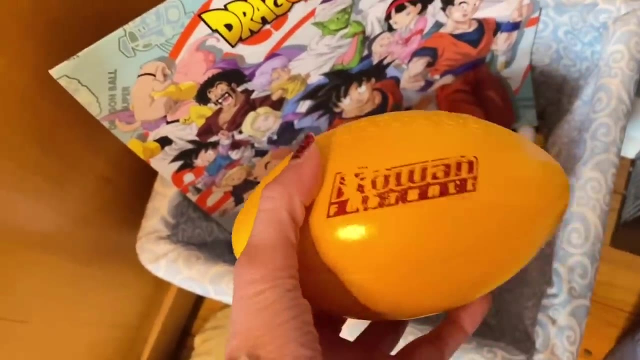 Well, we just got to clean up this last section and we're almost done. Now this poster is a keep. We're going to hang it on the wall. And the rest of this stuff? honestly, it can be. let go The basket. we can reuse it for organizing. 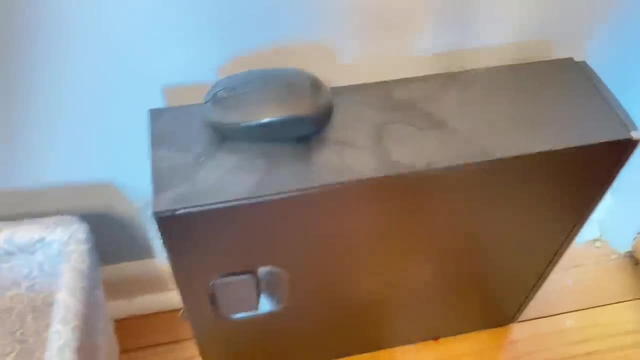 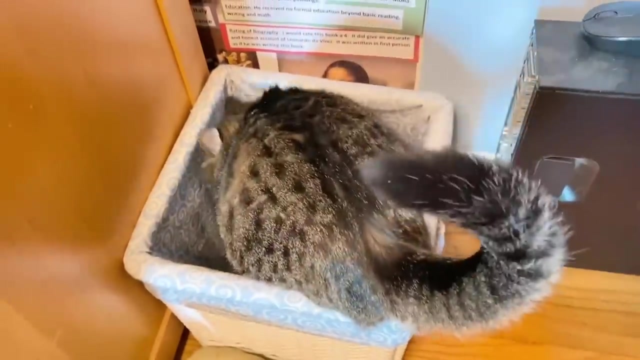 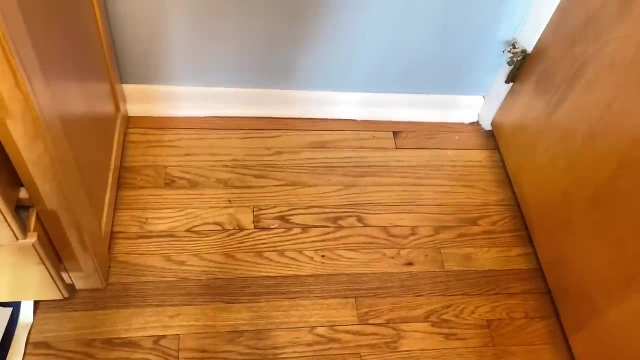 The pillow goes on his bed And this computer, I mean honestly, we really don't need it Now. this poster we can let go, and Miss Peppy has other plans for this basket. If she fits, then she shall sit Now. it was really important for me to clean out this little corner behind the door because 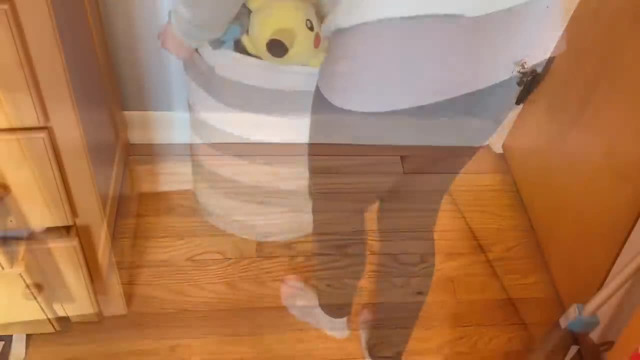 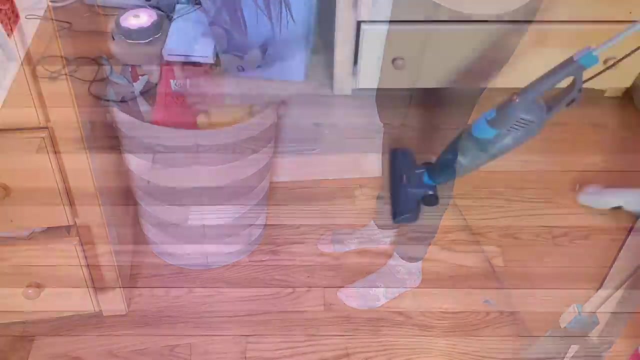 this is where I wanted to put Tyler Tyler's plushie bin. This is still a sentimental item for him, so I want to make sure that he can visually see where all his plushies are. And of course, my little tie guy is going to give a good vacuum on the floor. 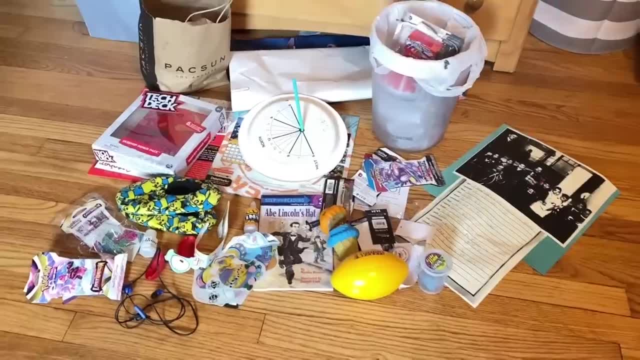 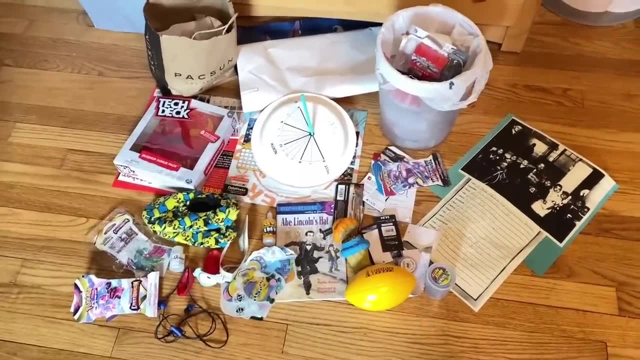 And I am very happy to say that this is Tyler's Tossy Tossy pile. Now there are things in the trash can and in the bag, and I just want to say how proud of him I am. Now Peppy is going to be a little bit more excited. 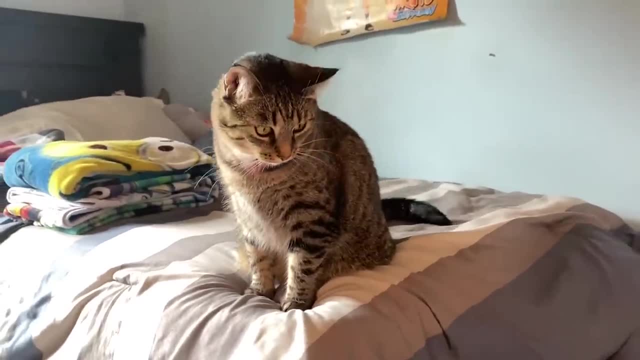 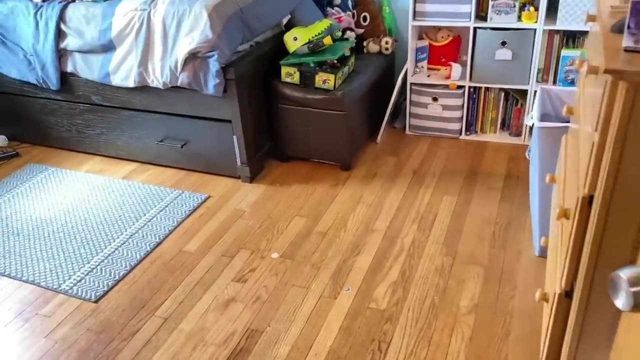 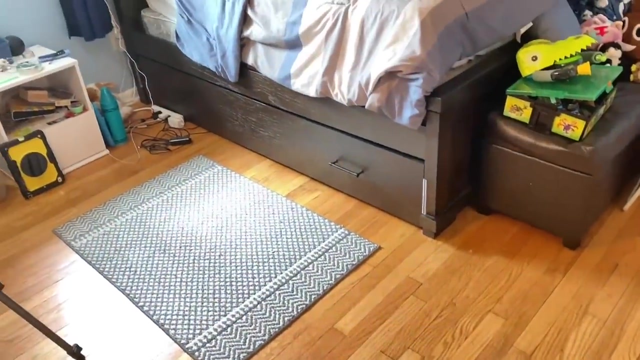 Now Peppy is giving her final looks to see if she approves of what has been done in this bedroom, And I'm happy to say that she approves. Tyler did a great job on decluttering, especially in this front section. when you first come. 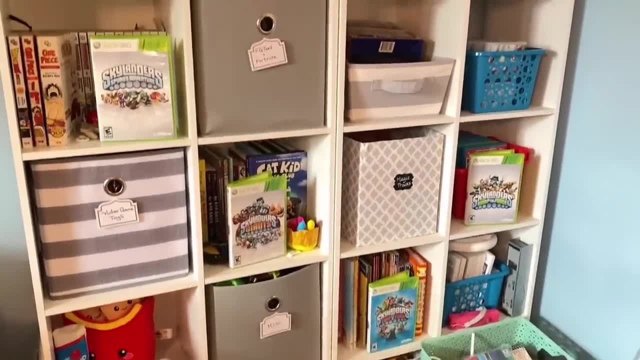 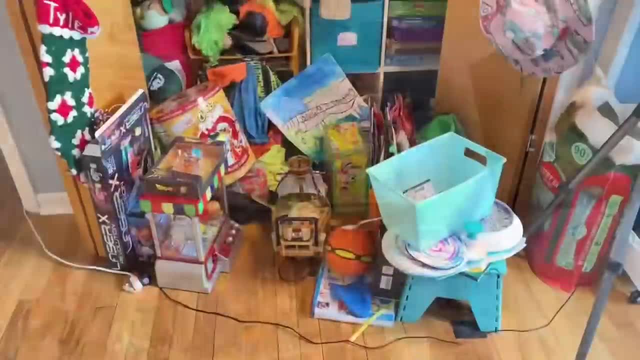 in. Now. we still have some work to do, like fully reorganizing this organizer so that he can be more successful at putting things away, And let's not forget this closet, because, yes, there's a bunch of stuff in front of. 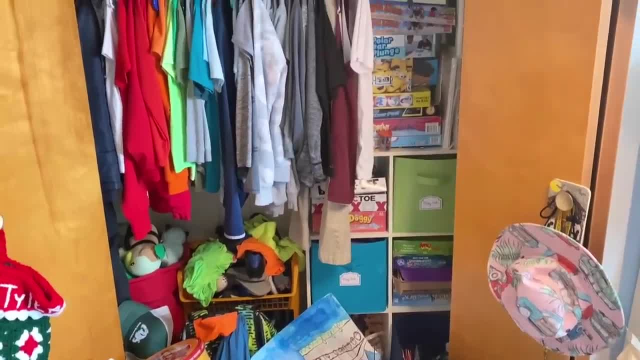 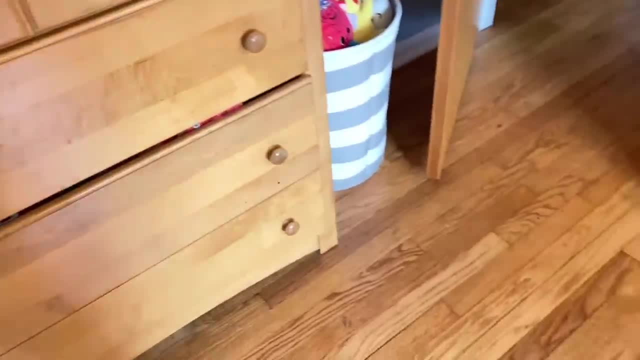 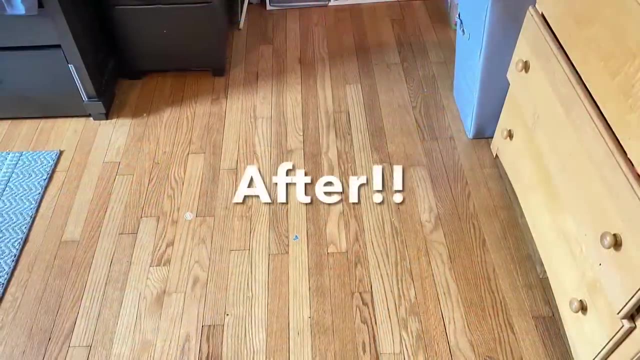 that, And this also needs to be fully organized as well, And in the month of March, we will be focusing on exactly that: organizing and resetting his room, because March is also his birthday month. So happy birthday to all of the March birthdays out there too. 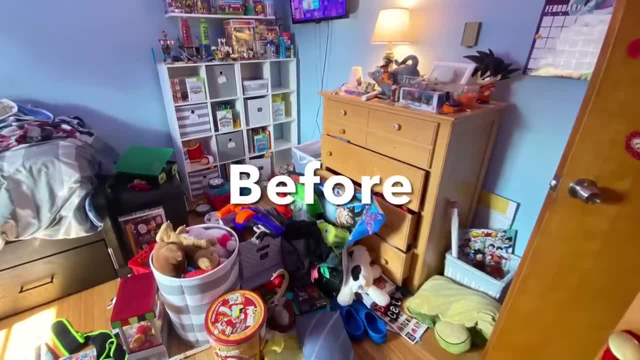 And my hope and my prayer is that this video motivated Tyler. I hope you enjoyed it. I hope you enjoyed it. I hope it motivated and encouraged you to declutter and clean something in your home today too.